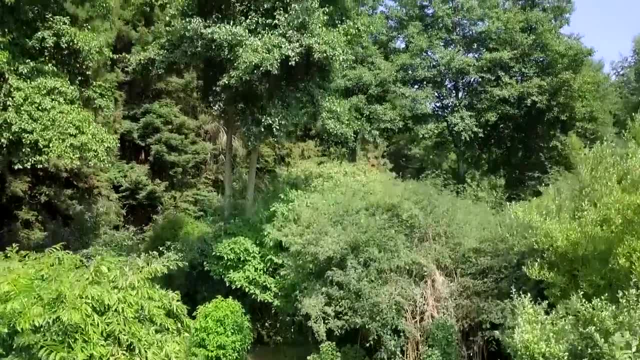 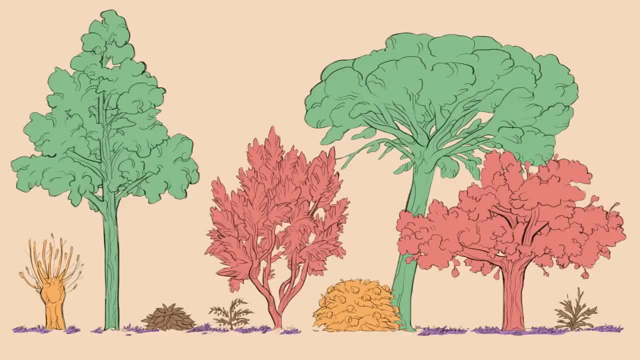 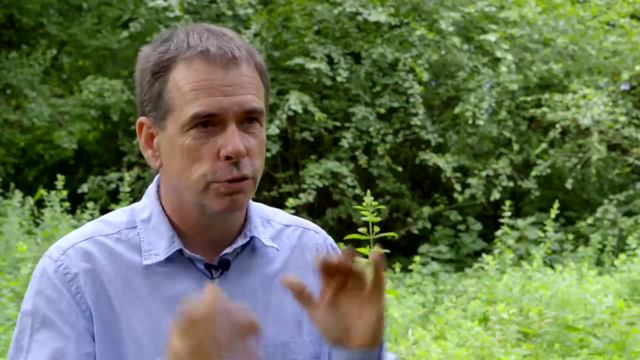 Forest gardens in a temperate climate tend to have seven layers or so: High trees, smaller trees, shrubs, perennials, ground cover layers, root crops and climbers. So it includes directly useful plants, many types of fruit trees, Common ones and much less common fruit trees. 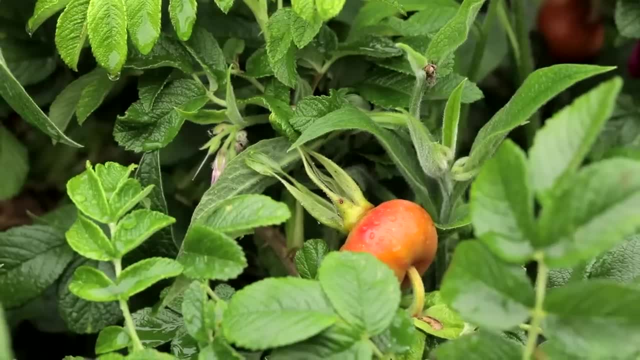 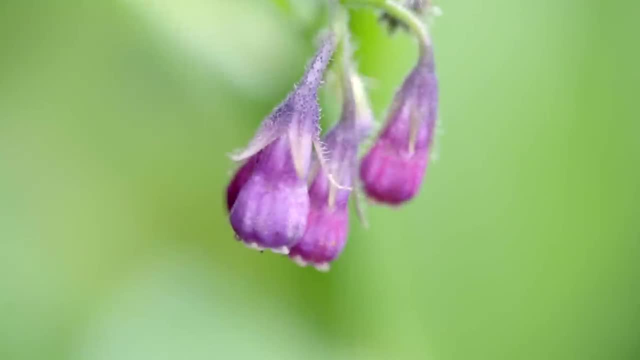 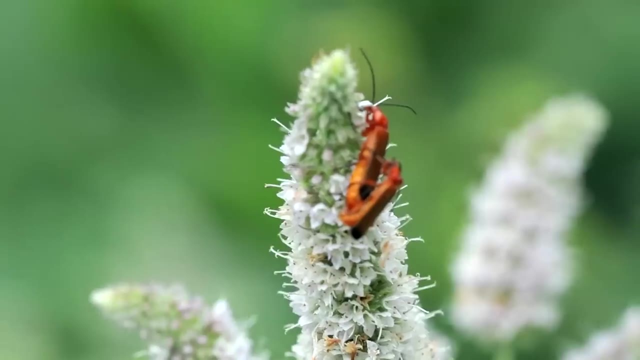 All the types of nuts, tuber crops, vegetables, medicinal plants, timber, but also logs that you might grow other things on, like mushrooms. There are also plants of indirect use system: plants to help the system function better, And that includes nitrogen fixing plants, mineral accumulators, plants to attract beneficial insects to eat all your pests. 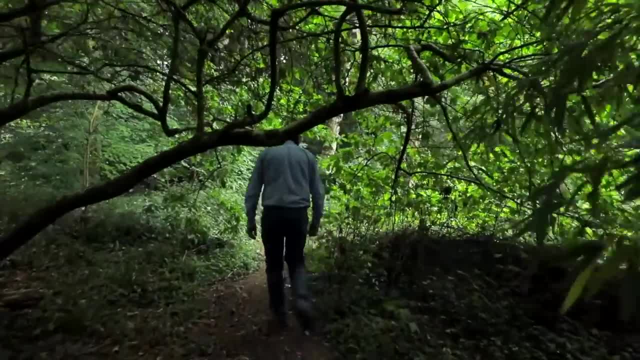 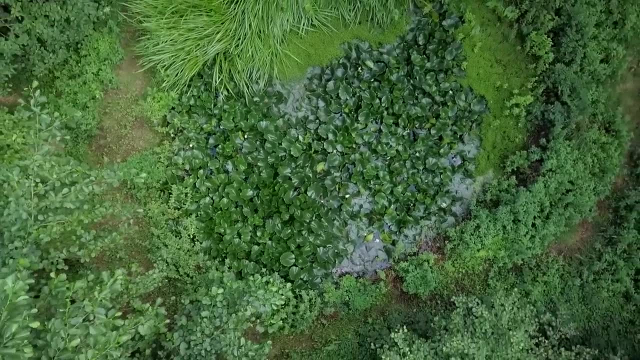 Forest gardens are very beautiful places to be in because, although they're managed, the management is light, So they have this very naturalistic feel And it is more like being out in nature than being in a cultivated garden. It can seem a bit overwhelming. 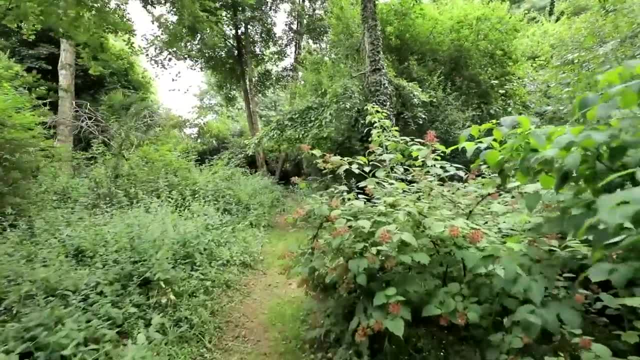 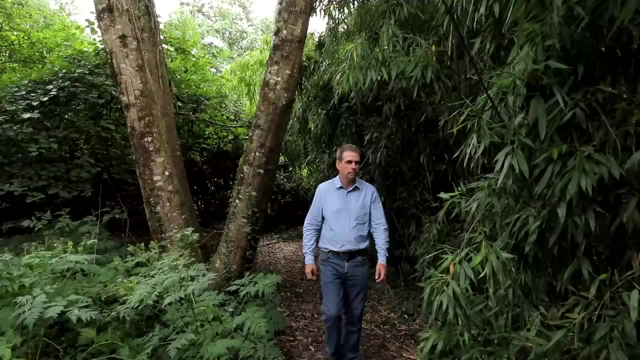 There's so many different species, You shouldn't let that stop you from beginning a project, because you don't have to know everything to begin with. Just start plant some trees and go from there. It's not the gradually increasing temperatures that damage plants. 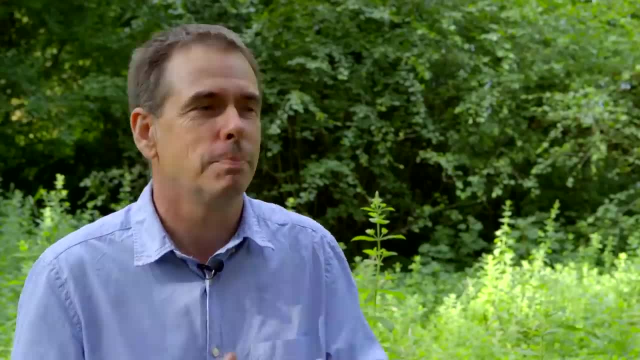 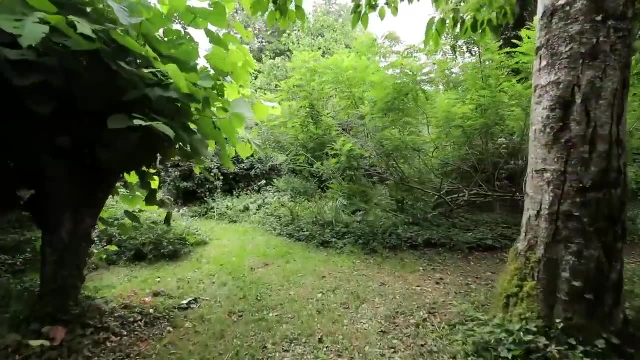 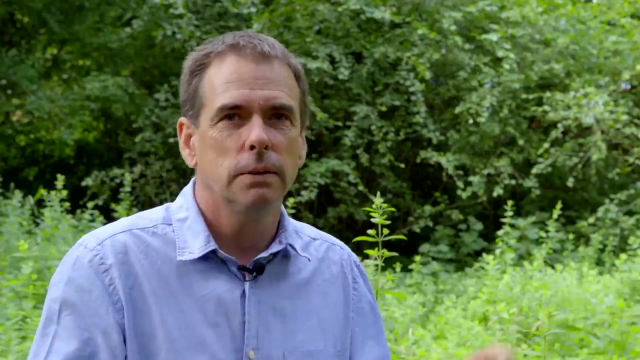 It's the increase in extreme events- Big storms, big winds, very heavy rain, hail, droughts. By having a very diverse system, whatever happens to the weather, most of your crops will probably do fine. Some may fail, some may do better. 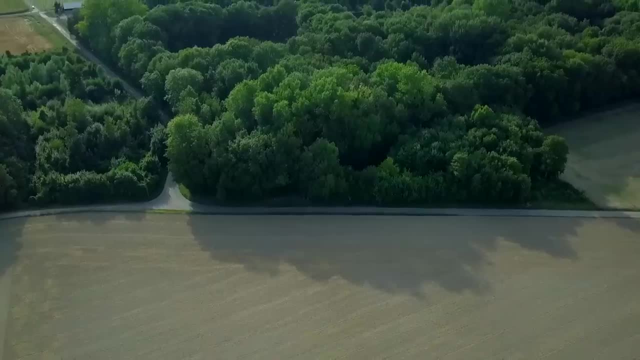 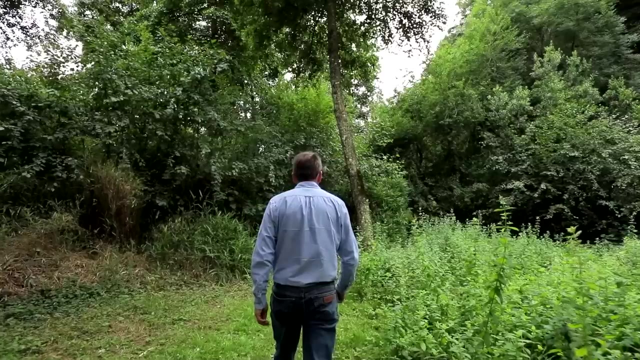 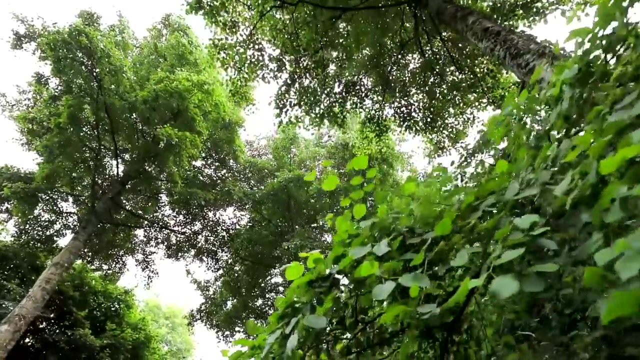 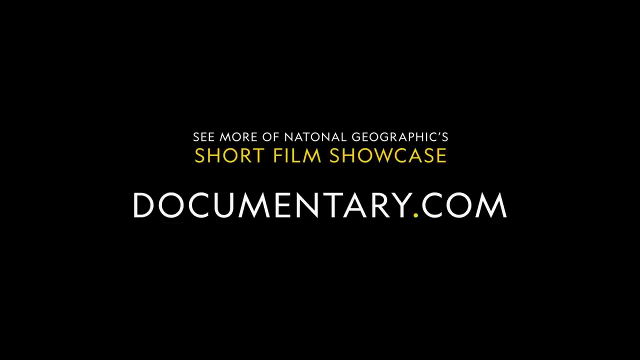 That's very important going into the future, because we don't know exactly what's going to happen to our weather. So by having a diverse system, it gives you maximum resilience. Taking care of ourselves is a key factor in our success. Well done, Birla. 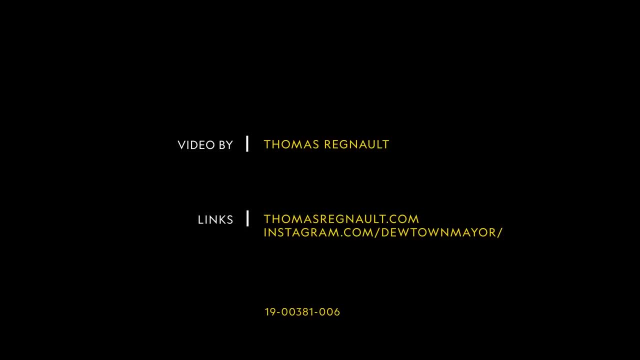 Thank you so much. Thanks, sir, For being so veryIES, and thank you for your patience. I appreciate it. Thank you, too. Thank you, Birla, You have a great day. Thank you, too, And thank you, Birla, for being so very honest about your interests. 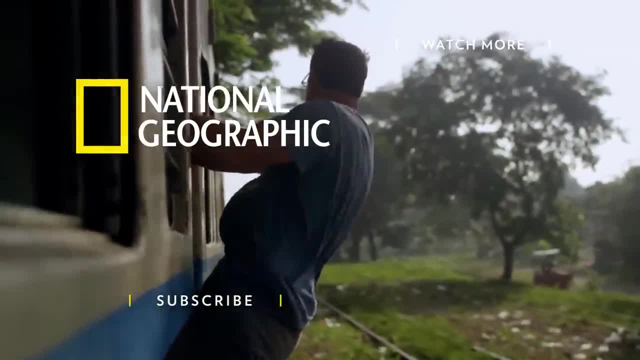 Thank you for talking with us. Thank you, Birla. That was a pleasure. That was a pleasure. Thank you so much And thank you, Birla. Thank you so much, Birla. Thank you Birla.